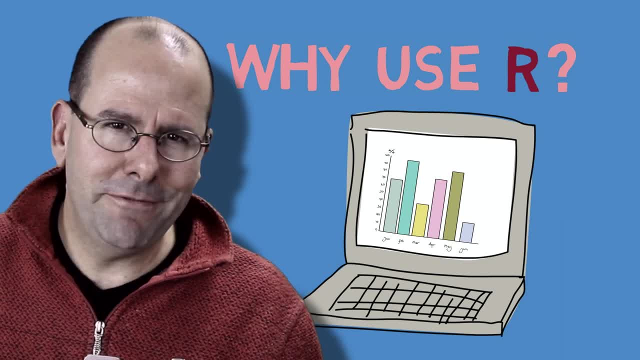 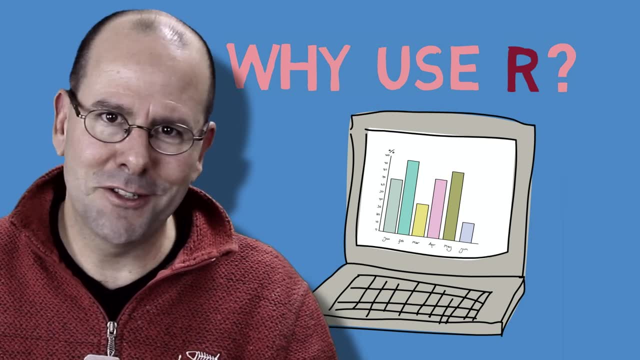 Now, R is essentially a programming language and you might find that fact a little bit intimidating or scary. but don't, And you'll see, when I do the little demonstration at the end of the video, that it's not difficult to use, that it's relatively intuitive and you can learn it. 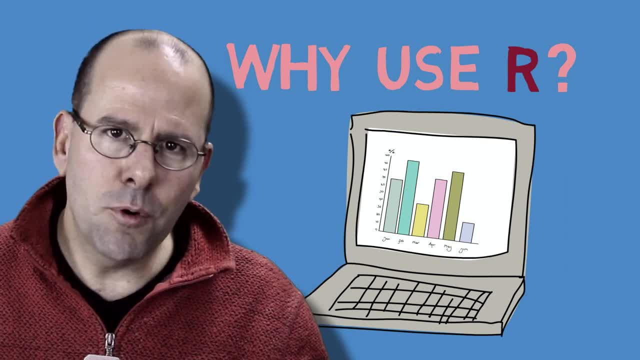 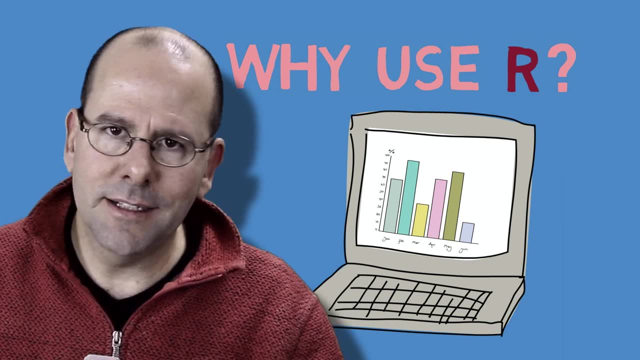 and there's loads and loads of support out there if you need it. The importance of using code when you do data analysis is that your analysis is reproducible. Somebody else can see exactly how it is that you got to the answers that you got to. Added to that. 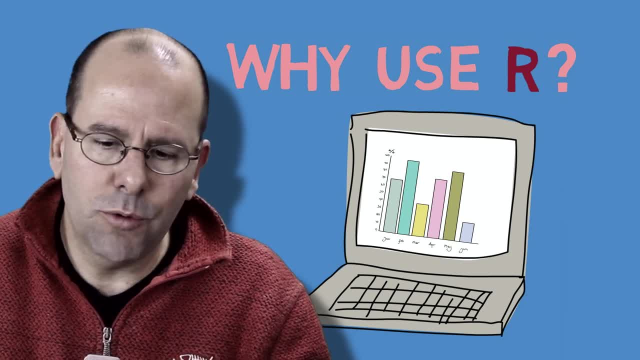 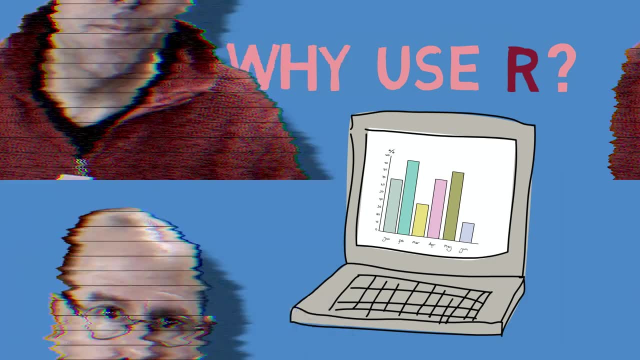 you've got the ability to collaborate with other people and they can look at what you've done and make suggestions or changes or identify mistakes in your analysis, and you can't do that with a point-and-click system. And the next reason why using code to do your analysis is important is: 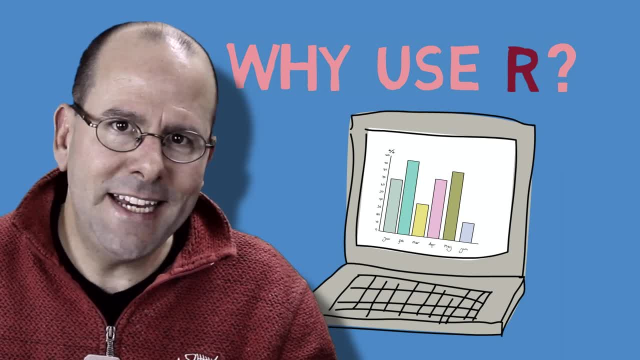 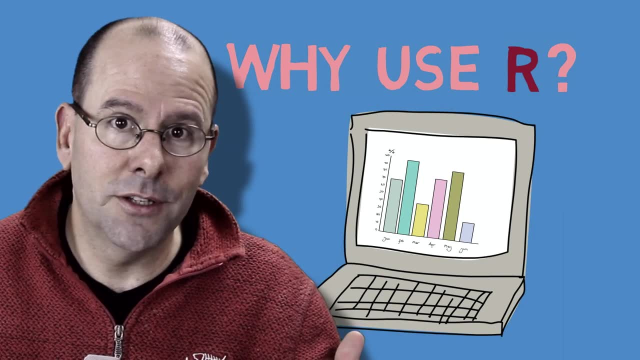 that not only is your analysis reproducible, but it's also repeatable. In other words, if a year from now you've got additional data- let's say you had data for 2018, in 2019 you've got double the data set. you want to rerun that analysis? you just run your code. 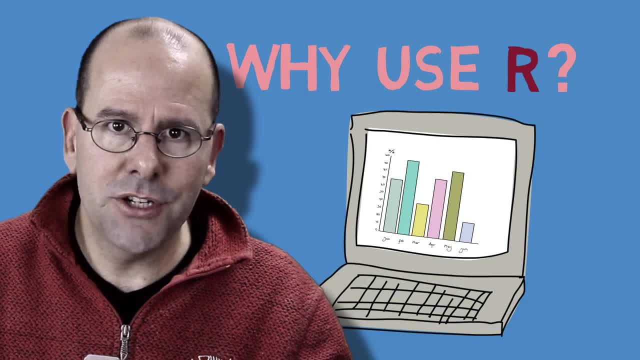 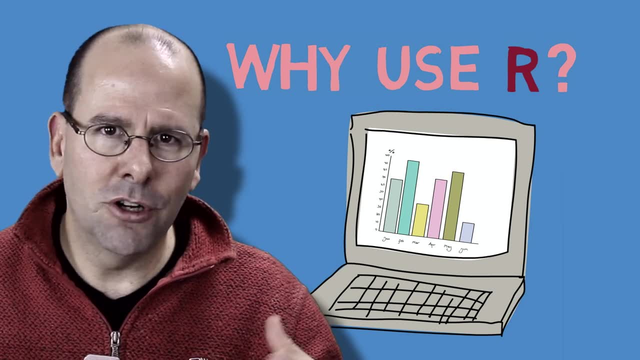 and everything- your data cleaning, your data manipulation and your analysis- all gets repeated right there and then at the push of a button. Now, one of the most exciting things about R is because it's open source. you've got people all over the world writing packages. 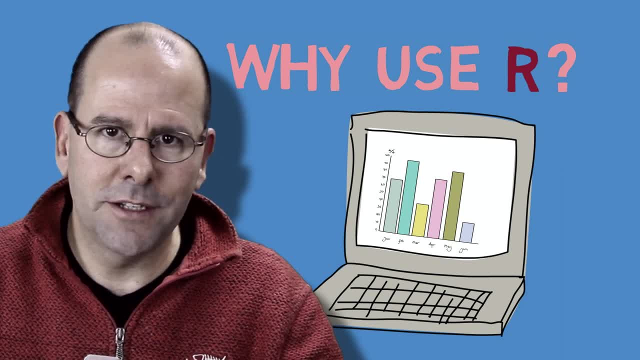 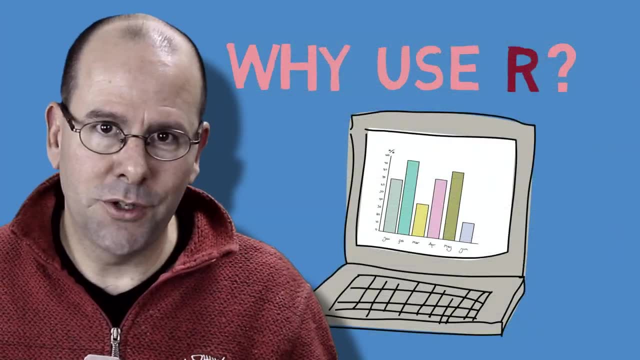 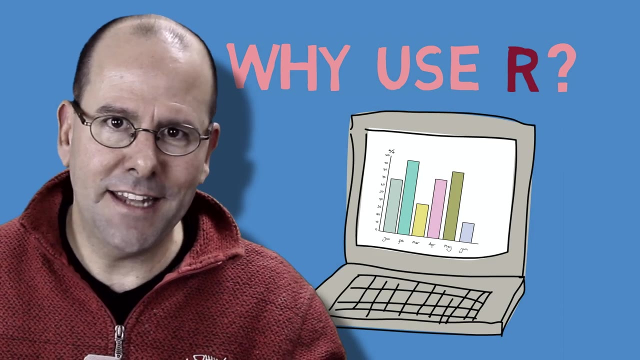 and packages are things that you can install and use that deal with very specific data analytic problems, And these are free, and there are literally thousands of them. Another big advantage of using R is that it has incredible data visualization and graphics capabilities. In fact, in that sense, it beats any other package. hands down, It's a slam dunk, nothing comes close. 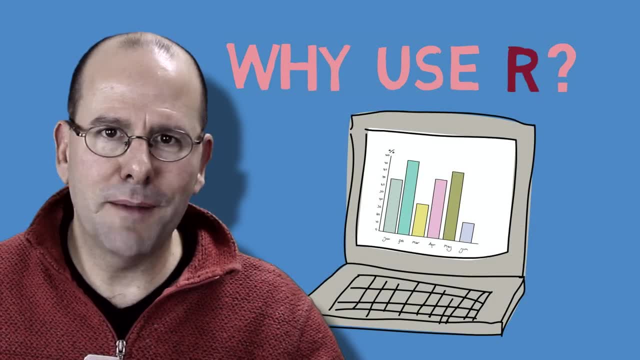 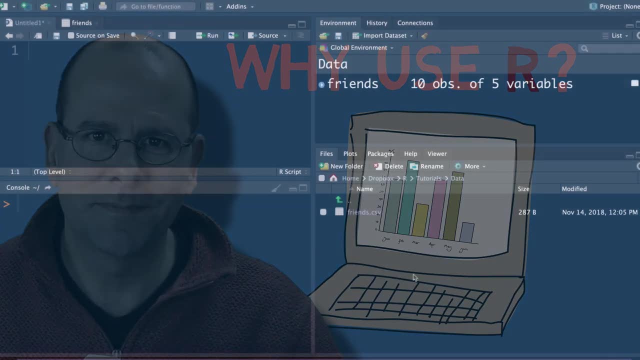 Right now I'm going to do a short demonstration just to show you that using a programming language to do analysis is not difficult, it's not scary, it's relatively simple. Okay, so watch this. Okay, so in this particular example, I have got a little data frame called Friends. I click on that. 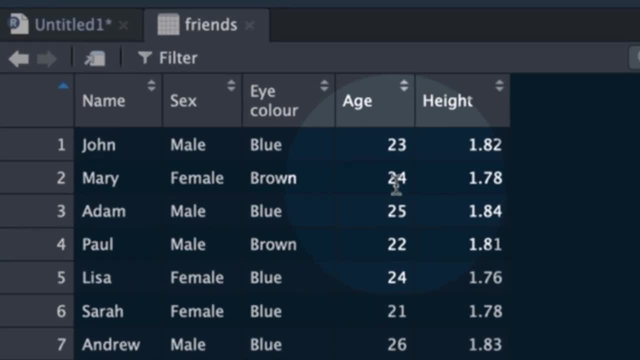 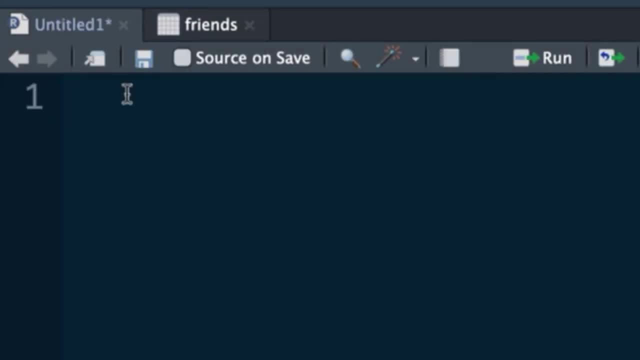 and we can see it over here. We've got some variables and some observations. I'm looking at age and height. Let's see what we can do with those. Basically, the way the coding works is you apply a function to an object. So in this case,